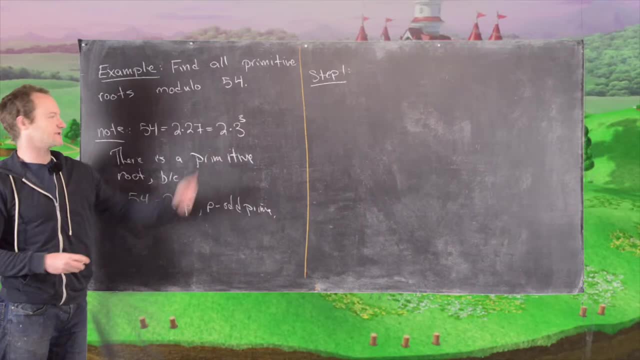 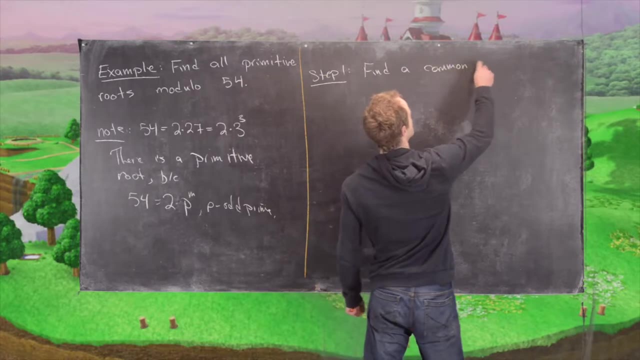 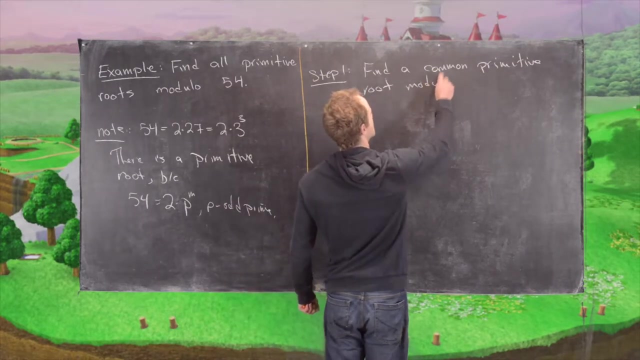 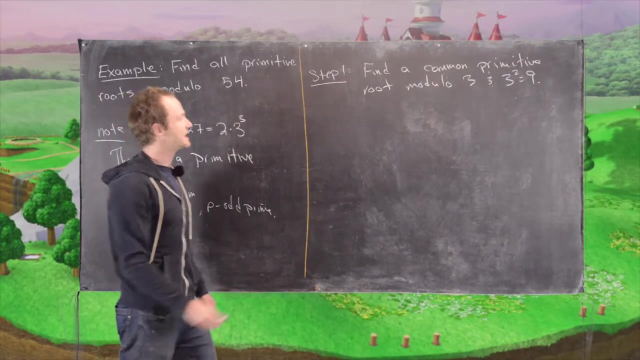 common primitive root modulo p and p squared. It just happened that here we have p equals 3.. So we want to find a common primitive root modulo 3 and 3 squared, which is obviously 9.. And it's easy to check here that 2 is this. 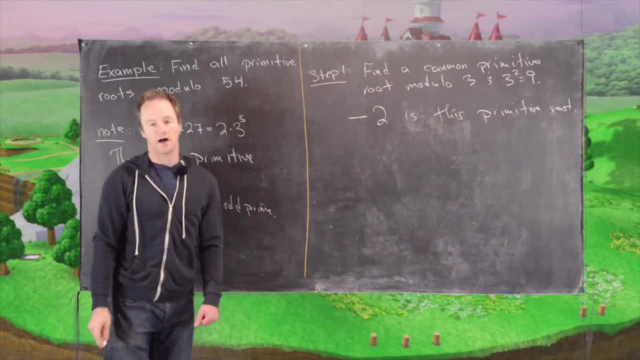 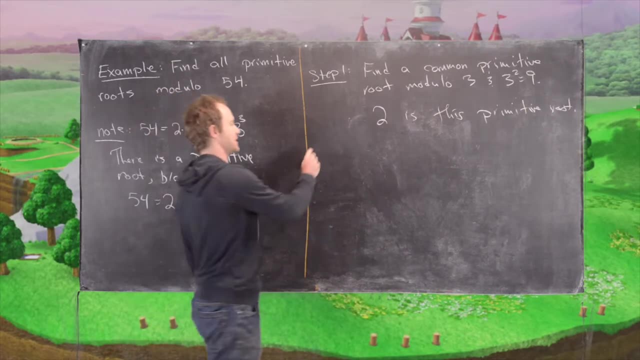 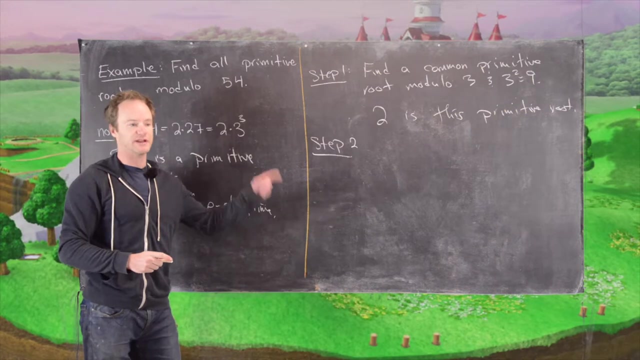 primitive root. Okay, so that looks like minus 2, but what I really mean is 2, is that primitive root? And so the next step is to ensure that this primitive root is written in an odd form, And so you know, since we're working modulo 3 or modulo 9,. 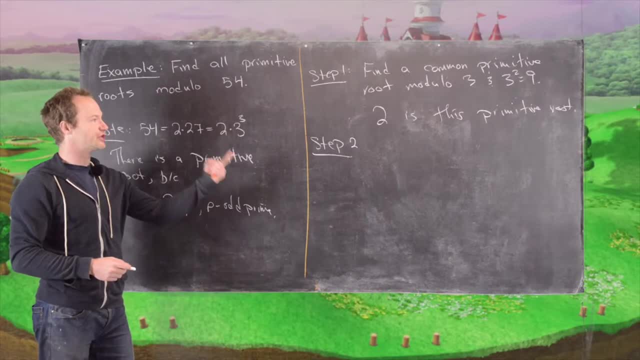 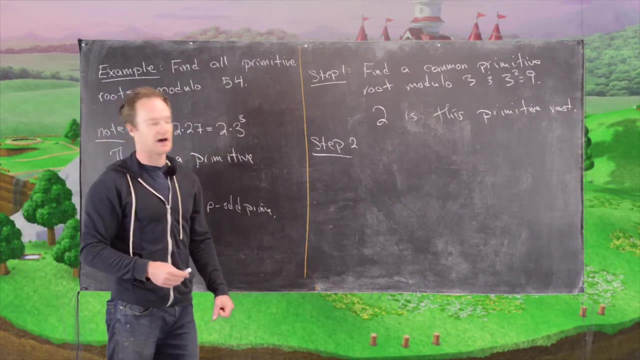 we can not just choose 2, but we can choose 2 plus 3 or 2 plus 9.. And that and that will work, And so we'll work 2 plus 9.. And so notice that 2 plus 9. 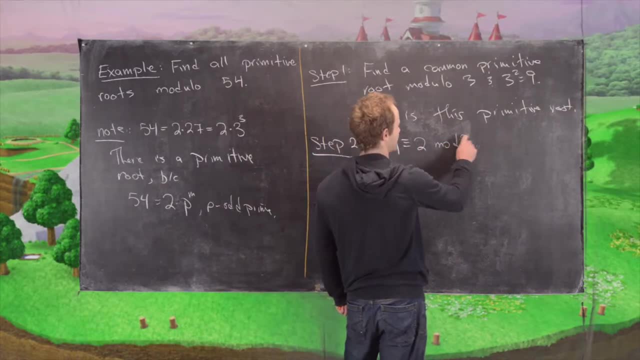 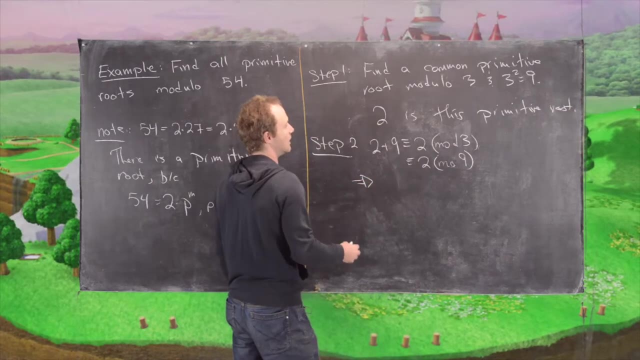 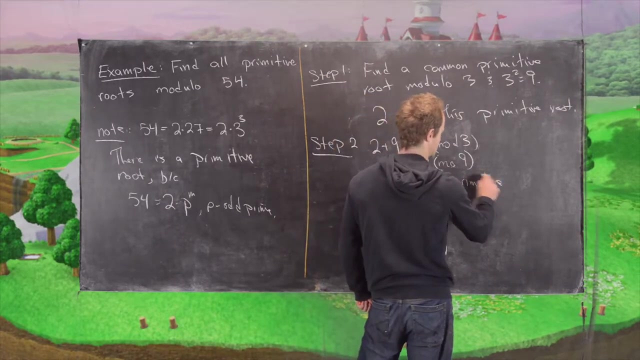 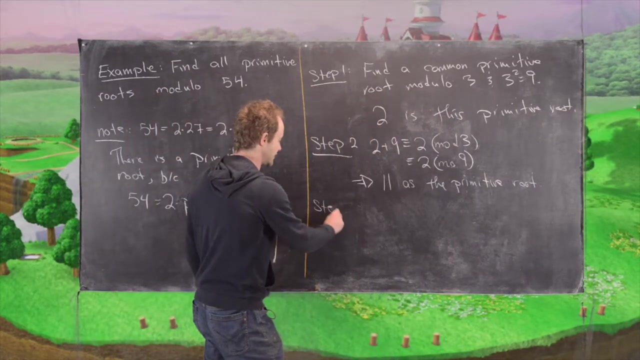 is congruent to 2 mod 3 and it's congruent to 2 mod 9.. So that means we'll choose 11 as the primitive root that we need. Great, And now we're actually all set. So step 3,. 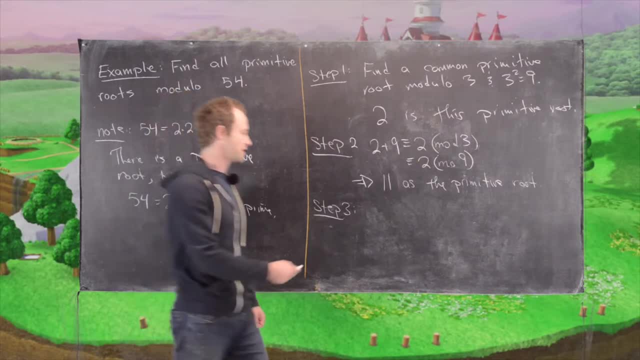 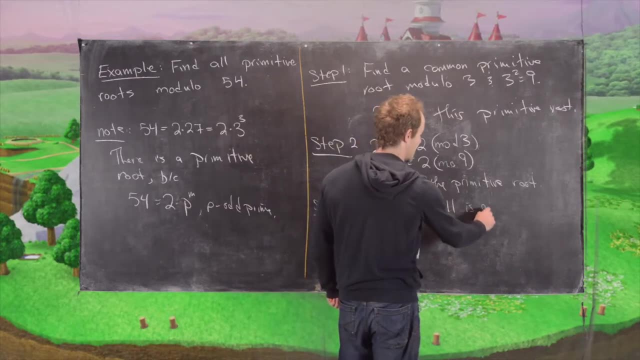 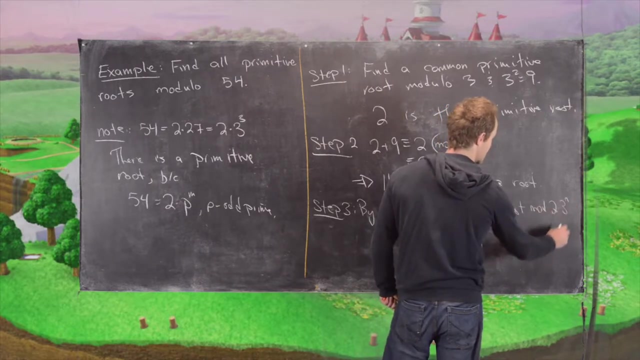 again using a proof of a previous result we have. so by previous we actually have. 11 is a primitive root mod 2 times 3 to the n, And this is for all n bigger than or equal to 1.. And so that includes. 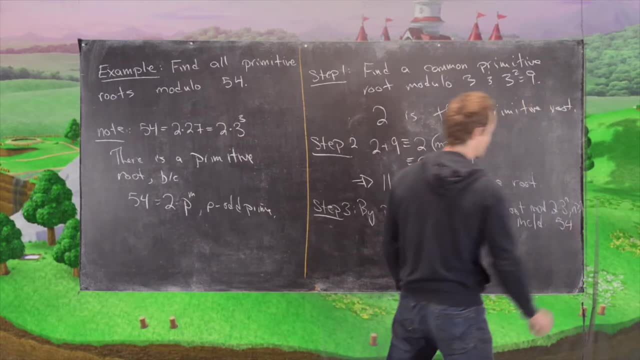 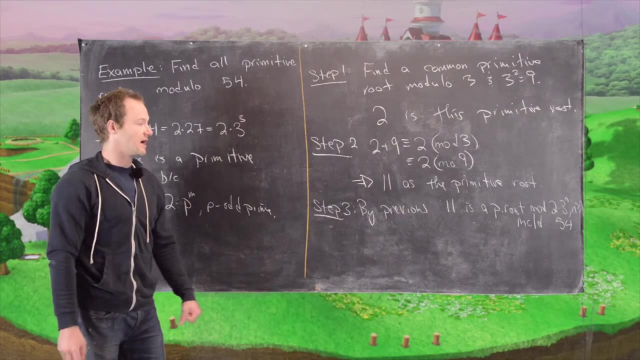 um 54,, which is 2 times 3 cubed. And so not only did we find a primitive root modulo 54, but 11 is a primitive root modulo 2 times 3 to the n for any n. Okay, So now the next step is the following: to find the rest of the primitive roots, So the remaining 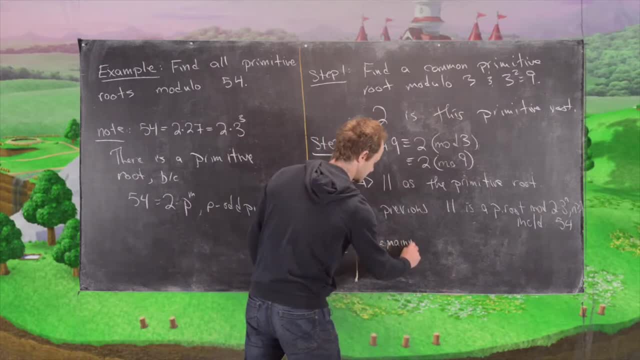 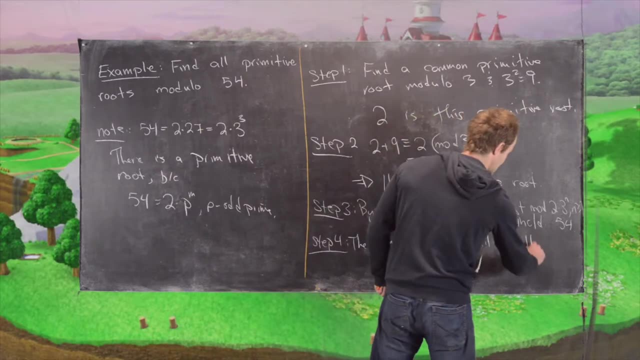 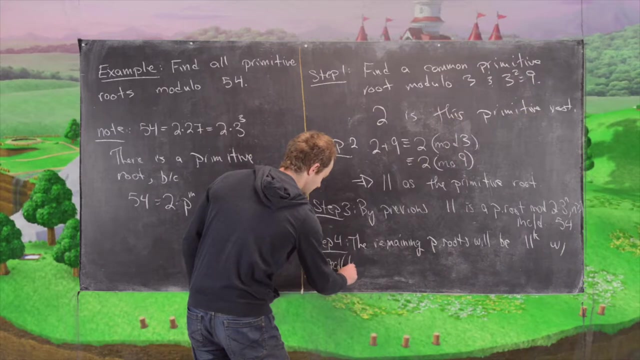 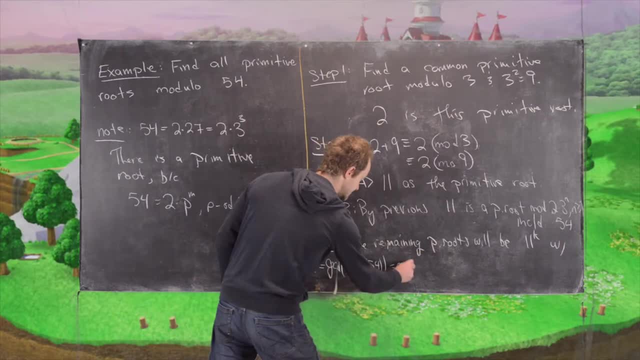 equals 1.. But that's the same thing at the GCD of k and 18.. You can check that phi of 54, 5 is 8,, 5 is 1, 5 is 1, 5 is 2 equals 2.. 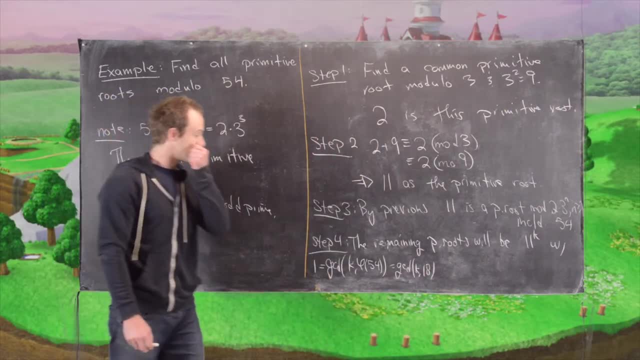 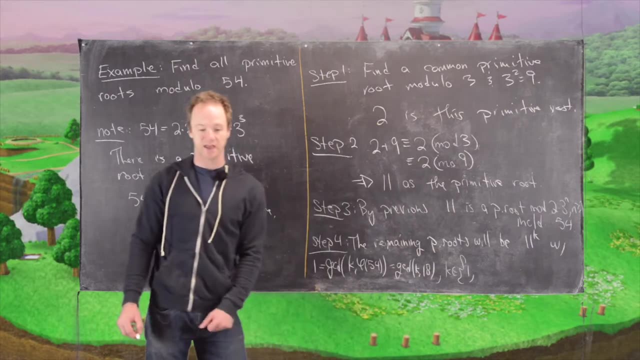 that phi of 54 is equal to 18.. So that tells us the following: So that tells us: we have k in the following set, One, so we can't use two, three or four, So we have five, seven. 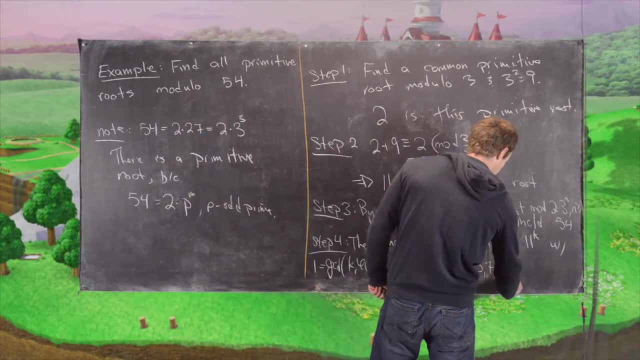 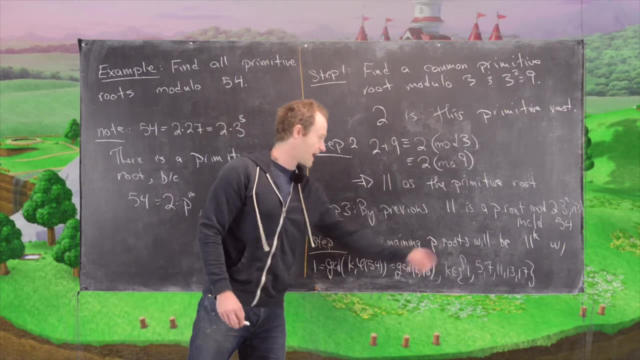 We can't use eight, nine or 10. And then we have 11,, 13, and 17.. So in the end we have k in this set. So I'll clean up the board and then we'll finish this off. 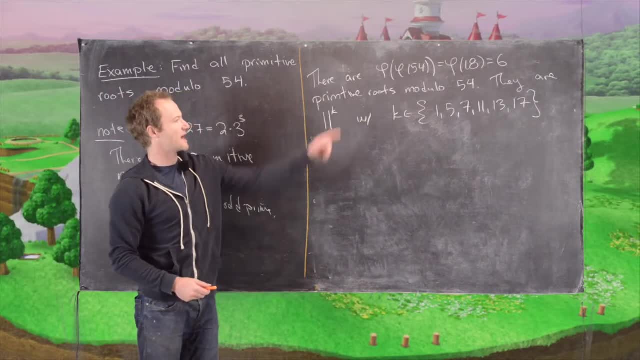 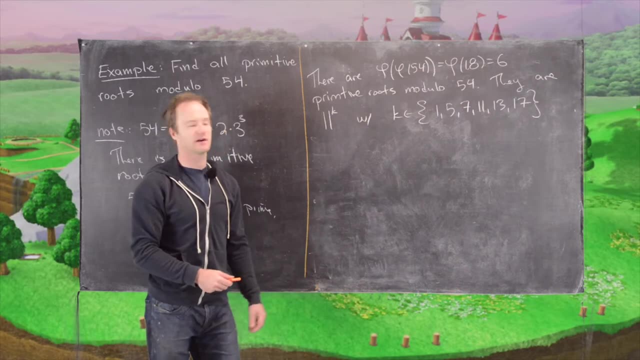 Okay, so picking up where we left off. So let's recall that we have all the primitive roots of modulo 54 are 11 to the k, where k is in the set one, five, seven, 11,, 13, and 17.. 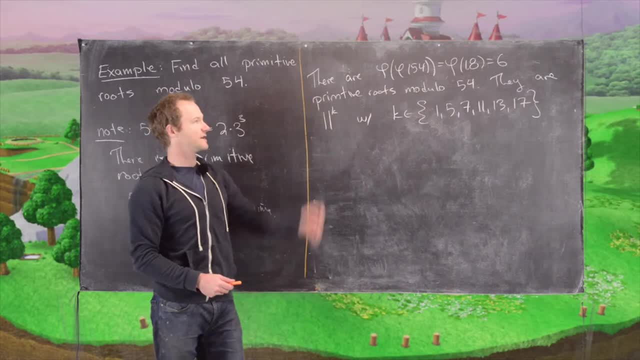 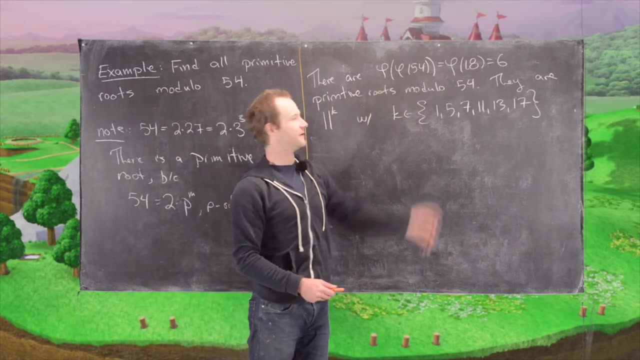 So notice, there's six elements in that set And then by a previous result, we know that if there's a single primitive root, modulo 54, then there are phi of phi of 54. In other words, phi of 18, which is six primitive roots modulo 54.. 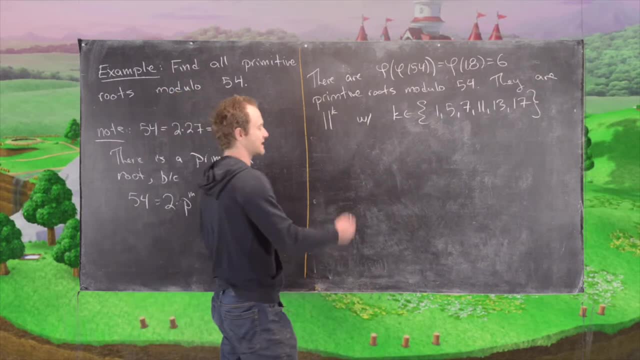 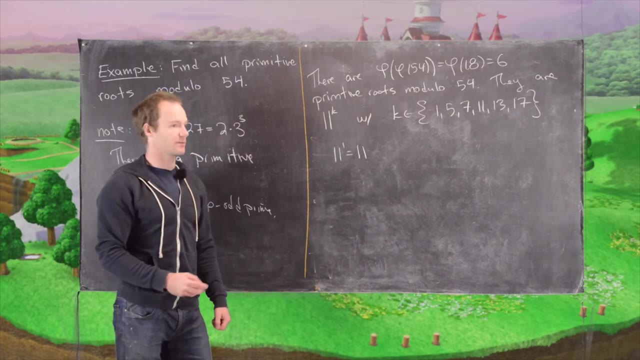 So that indeed, will find all six of them, And so now we can calculate all of these numbers. So 11 to the one is obviously 11.. Now I'm gonna leave off the calculation, but you can look at previous videos for how to quickly calculate this arithmetic modulo 54.. 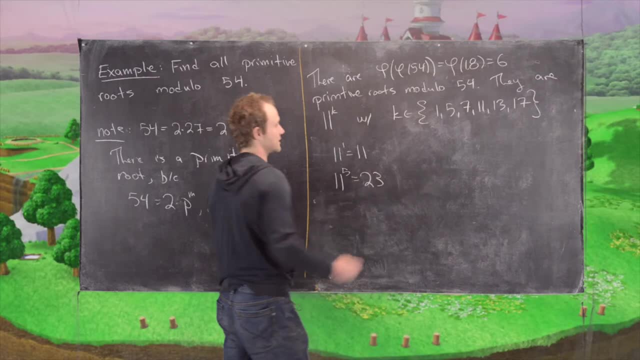 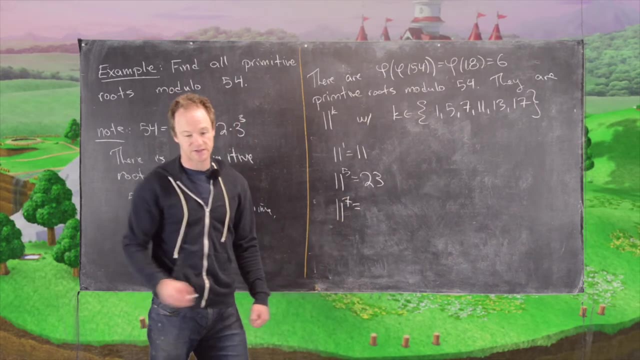 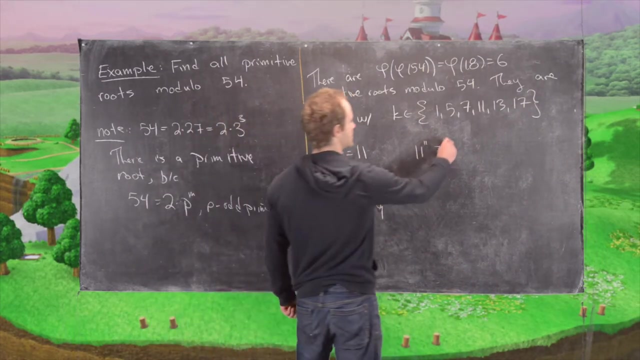 And then 11 to the five is 23.. And here we're working mod 54 the whole time. 11 to the seven is 29.. 11 to the 11 is 41.. 11 to the 13 is 47..